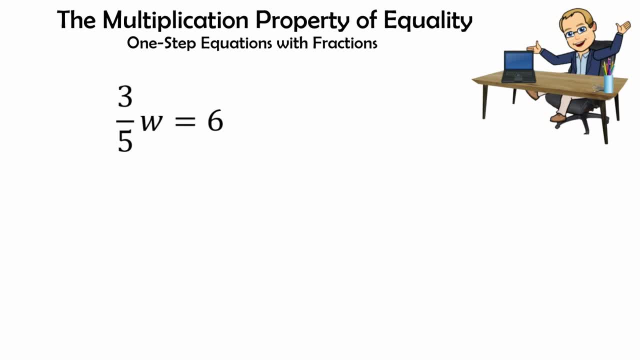 multiplication property of equality, which means, whatever I do on the left side, I am going to make this equation equal. I'm going to do the same on the right side. So when we have 3 over 5, when we have 3 over 5, that means that we are going to multiply it by its reciprocal of 5. 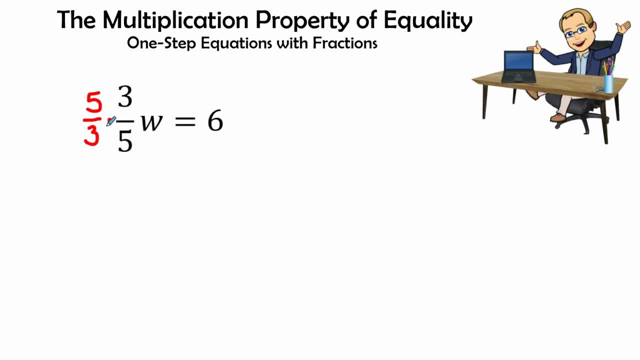 over 3.. Now, because I do it on the left side, I'm going to have to multiply by 5 over 3 on the right side. Now, this 6 is a whole number and to make it equivalent as a fraction, I'm going to make that 6 over 1.. So now that I can either do one of two, 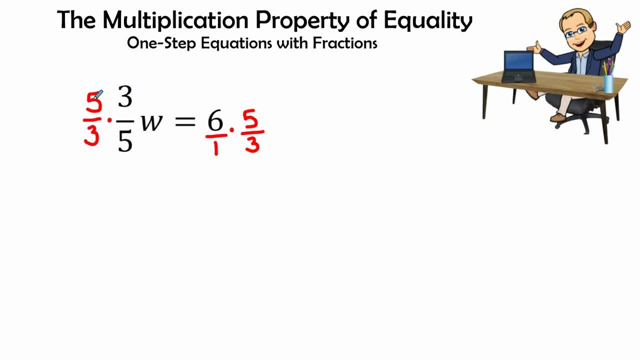 things. I can multiply across: 15 over 5 times 3 is 15, and 3 times 5 is 15.. So 15 over 15 is equal to 1.. Therefore I'll have one w and I would have my variable by itself, But another way I can do it. 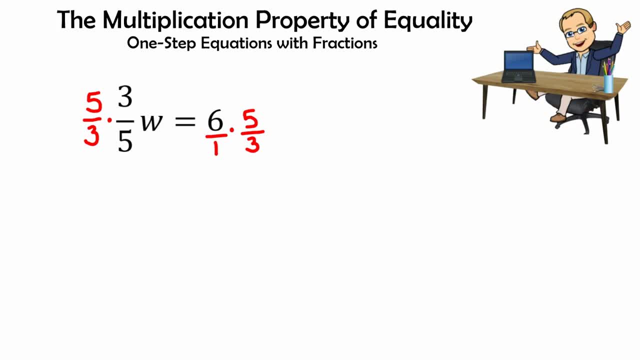 is by multiplying or cross-canceling. And in cross-canceling I'm going to go ahead and say the 5 goes into the 5 one time and the 3 will go into the 3 one time, because they're factors of. 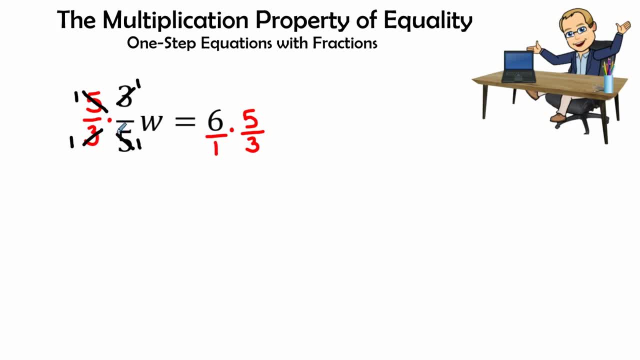 each other. They're the same number, So through the identity property they are the same. Therefore 1 times 1, and 1 times 1 gives me 1 over 1.. So that gives me w by itself Now 6 times 5,. 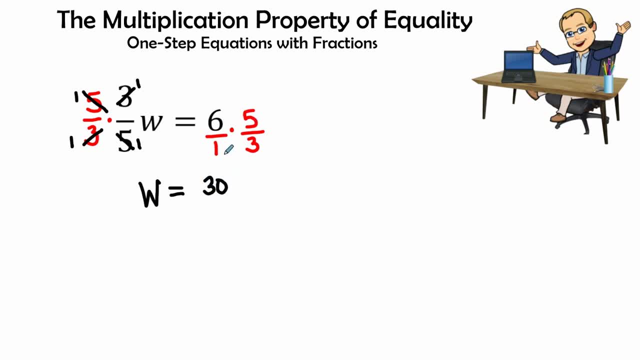 on the right-hand side will equal 30. And 1 times 3 in the denominator would be 3.. Now if I simplified 30,, how many times does 3 go into 30?? And the answer is 10 times. So my correct answer. 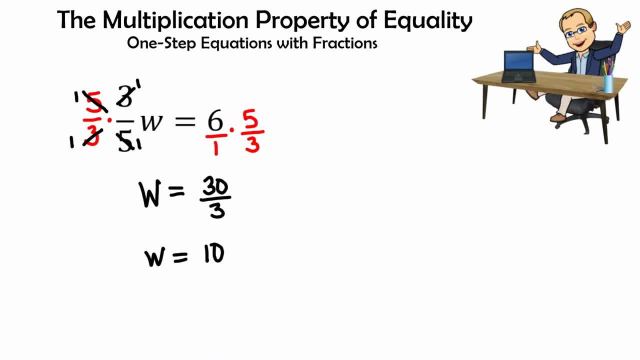 is w equals 10.. Let's go ahead and give that another shot, another try with another sample problem. Here we go. I have something hidden right here for you. So our next one is: 7 eighths t equals 14.. Now, when I get rid of this fraction, I'm going to